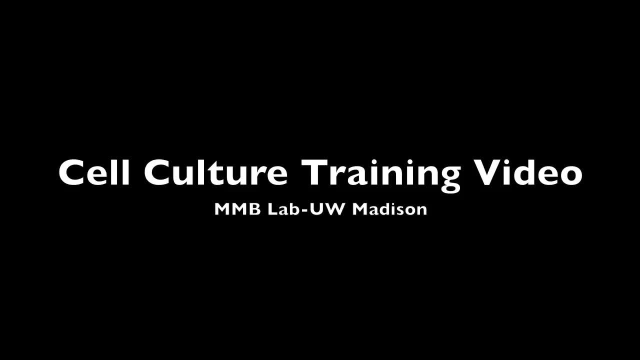 Welcome to the MMB Lab cell culture training video. A successful cell culture depends on various things: laboratory equipment, the quality of the reagents and cells you use and your sterile techniques. Let's start by looking at the equipment inside the MMB cell culture room. 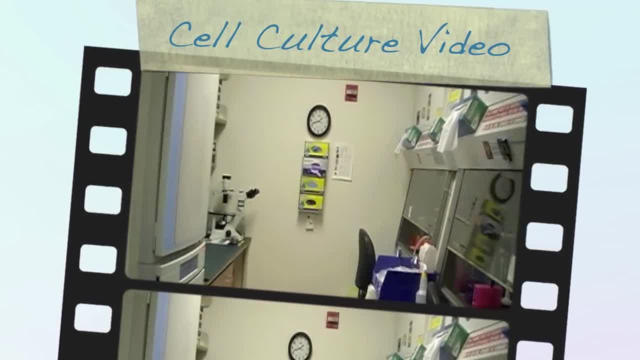 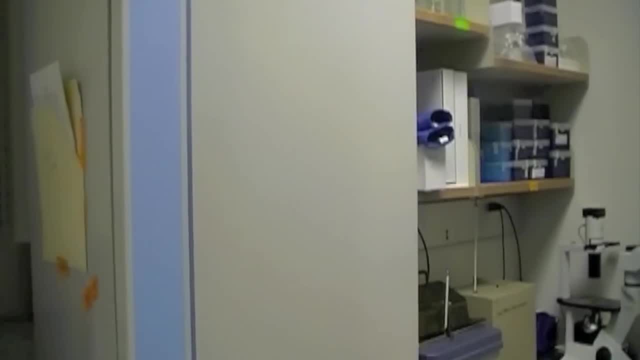 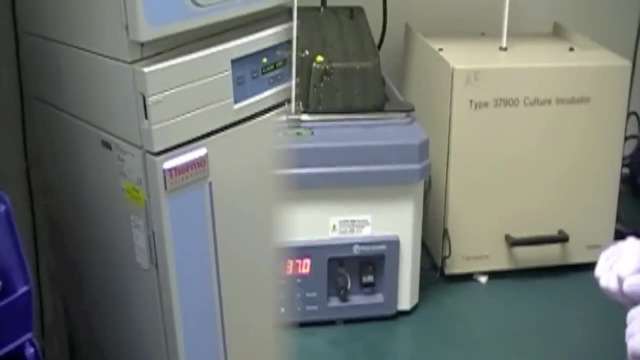 As you come inside the cell culture room, you will find two sterile incubators that are used to keep the cells at 37°C and 5% CO2.. The top incubator is used to maintain cell cultures in petri dishes, flasks, and the bottom incubator is reserved for microchannel cell cultures. 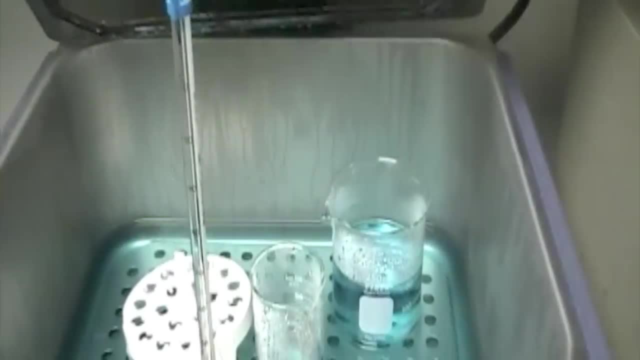 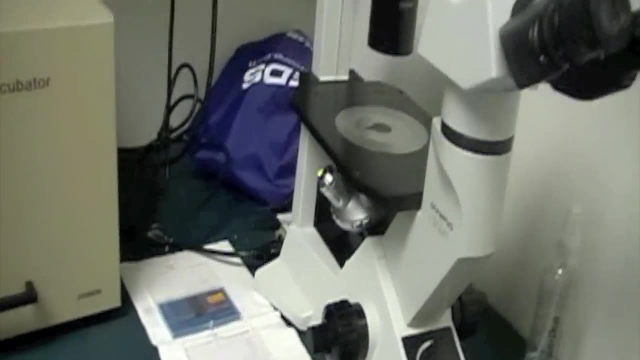 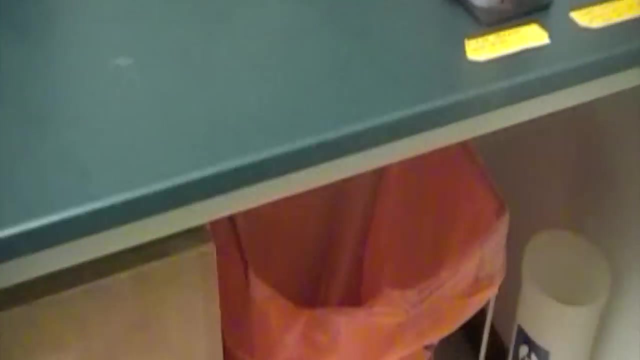 Right next to the incubators, you will find a water bath at 37°C used to warm up your cell reagents. You will also find a microscope and two hemoglobin tubes. You will also find two monocytometers to help you with cell counting, an orange bag used to dispose of cell-containing flasks or tubes. 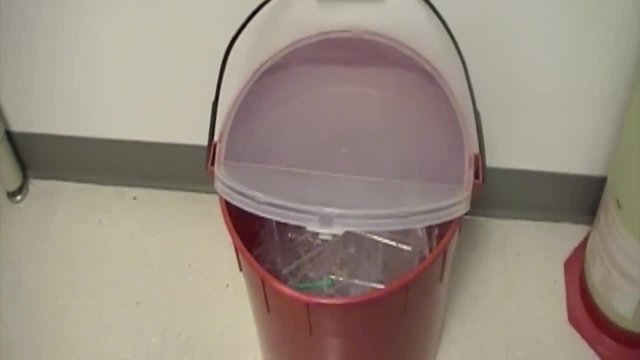 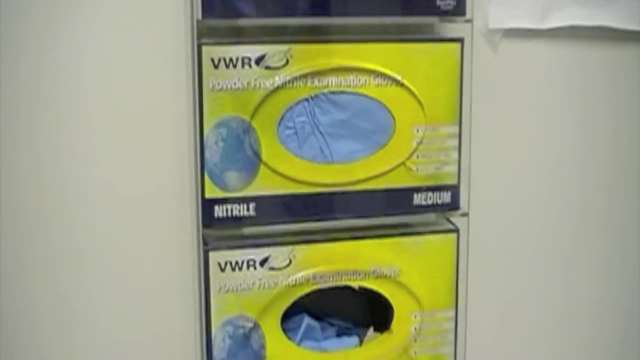 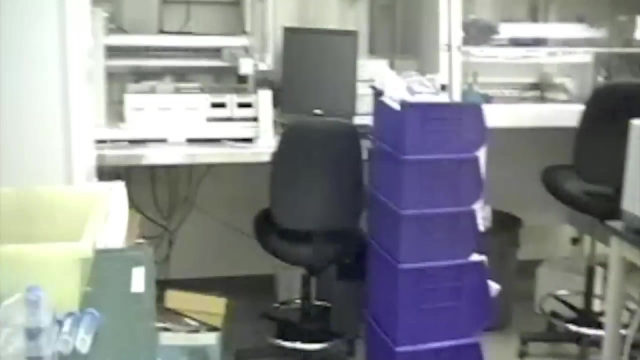 an orange basket to dispose of glass pasture pipettes containing cell waste, a cardboard box to dispose of regular glass pipettes and a plastic tube to dispose of glass pipettes used with cells. On that wall you will also find gloves of different sizes. 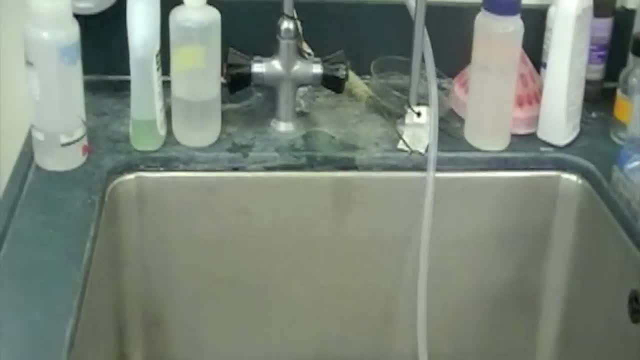 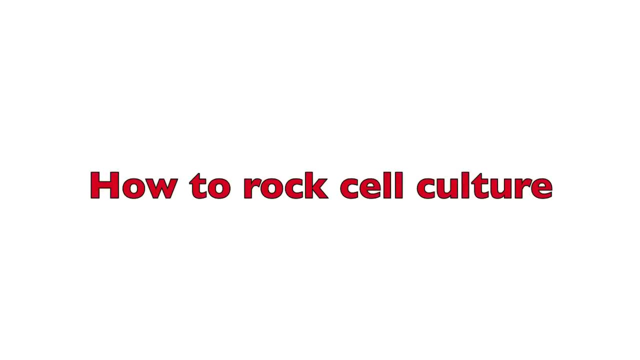 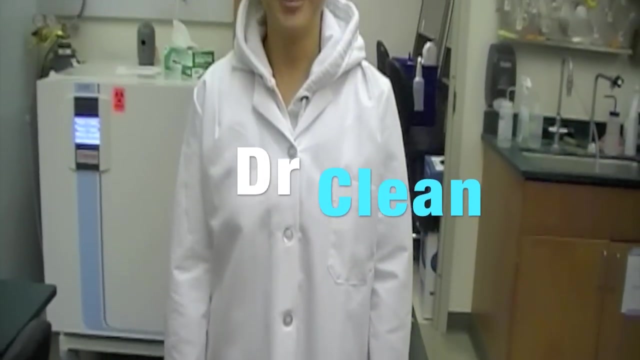 Outside of the cell culture room, we have a sink for cleaning up and bleaching your cells. Now, for the purpose of teaching you how to pass cells using proper sterile techniques, we will follow Dr Klin's techniques. Notice that Dr Klin is wearing closed-toed shoes, long pants, a lab coat, goggles and, yes, a huge smile. 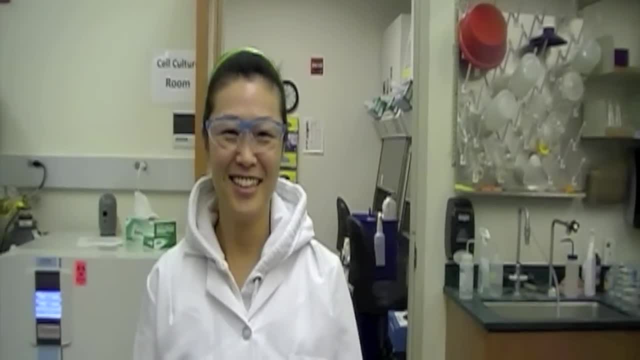 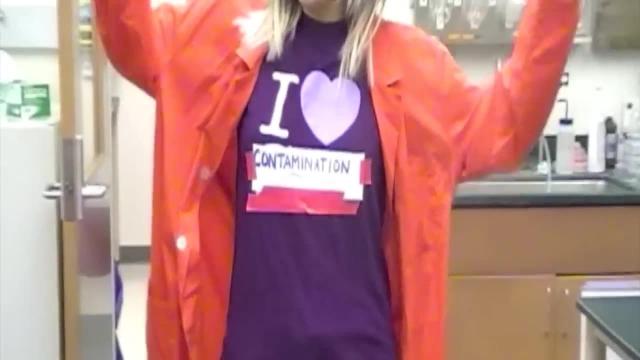 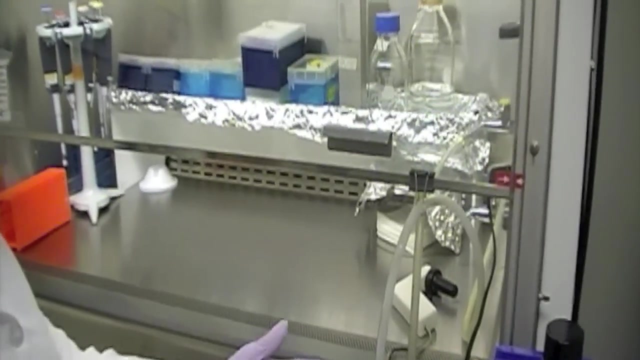 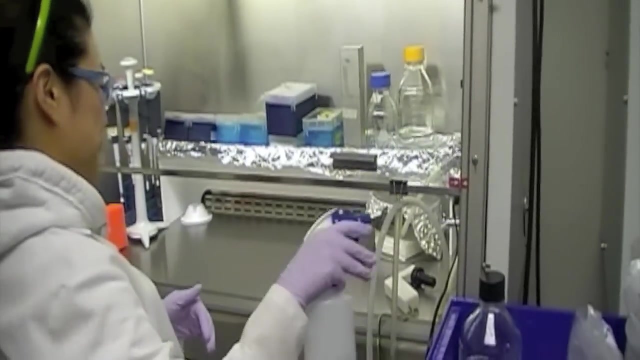 Go Dr Klin And of course we will avoid doing things like doctor contamination. I'm sexy and I know it. Okay, so let's see how Dr Klin performs a clean and sterile cell passage. First, Dr Klin puts on clean gloves, sprayed her hands with 70% ethanol and sprayed and wiped the inside surface of the bio cabinet with ethanol. 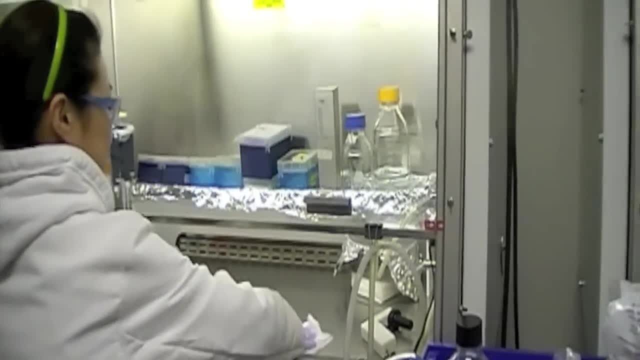 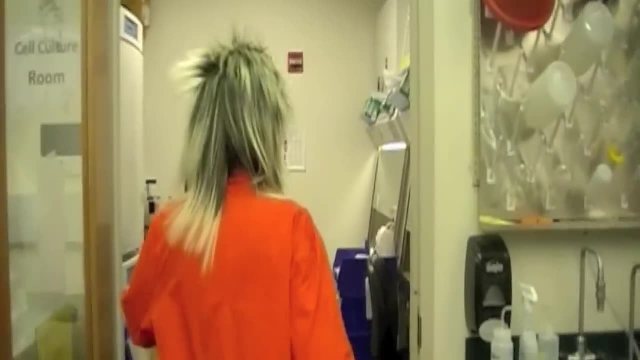 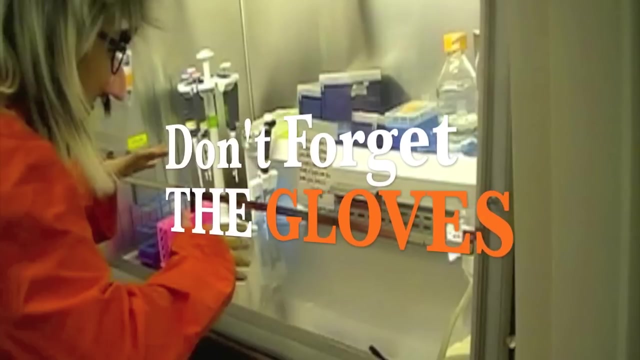 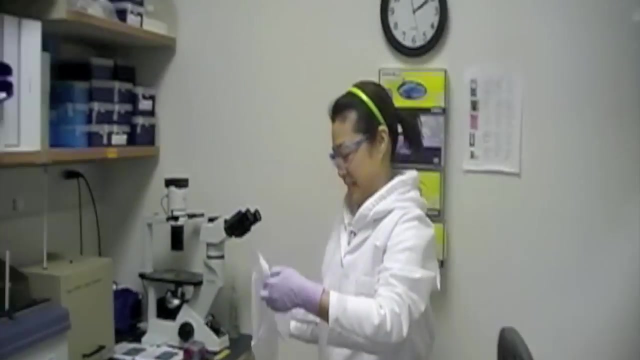 Mmm, very clean. Let's see how Dr Contamination is doing. Hey, Dr Contamination, you need to wear gloves, Don't Too bad, Dr Contamination, too bad. Okay, so going back to Dr Klin's sterile techniques, the next step is to get your reagents from the water bath. 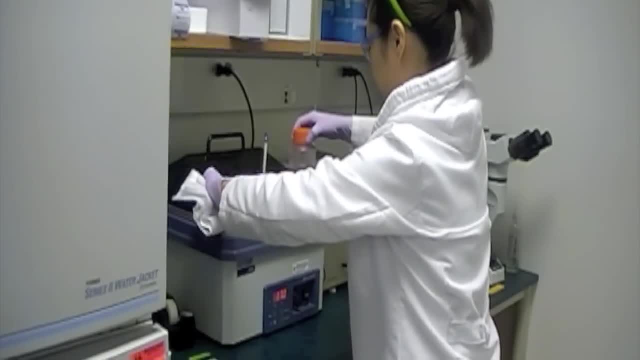 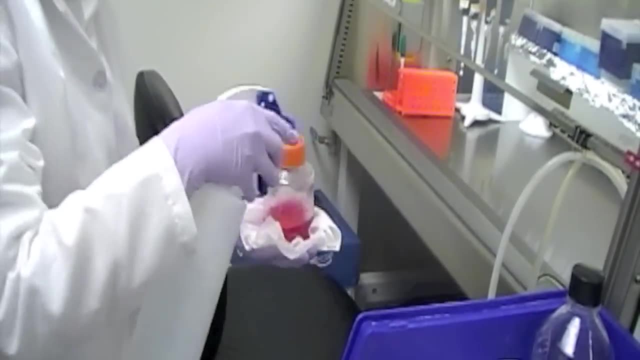 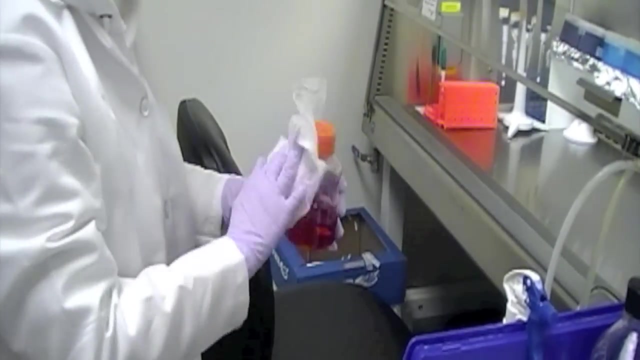 Notice how careful Dr Klin is when handling the media bottle. It is always a good sterile technique to avoid tilting your media bottle, since the media accumulated in the lid can be a possible source of contamination. Also, notice how she sprays and wipes all the bottles with ethanol before placing them inside the bio cabinet hood. 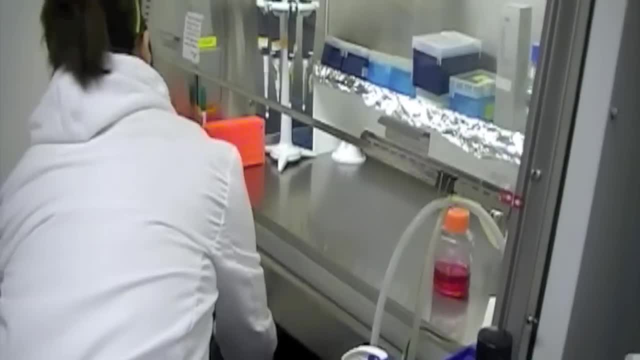 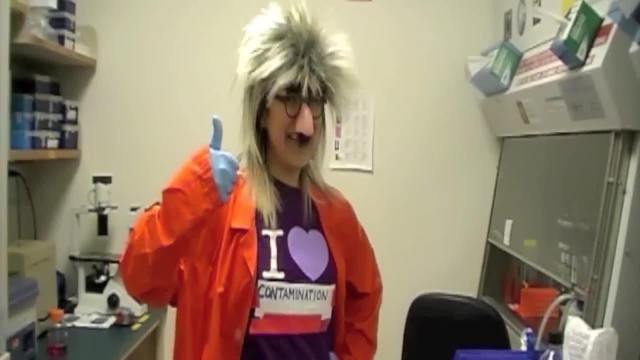 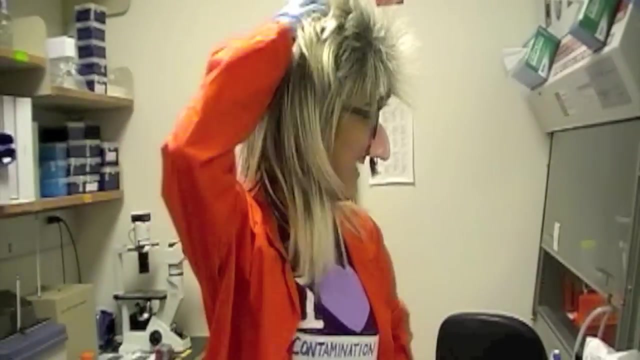 Everything that goes inside the hood needs to be sprayed down On the other side, Dr Contamination. Oh no, you have a mess inside your bio cabinet, Dr Contamination, And no, Don't spray. Scratch your head with your hands. 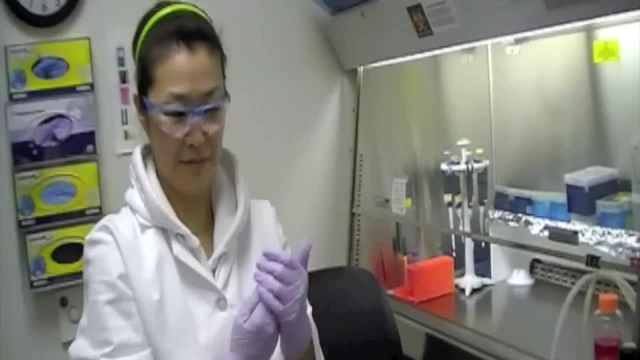 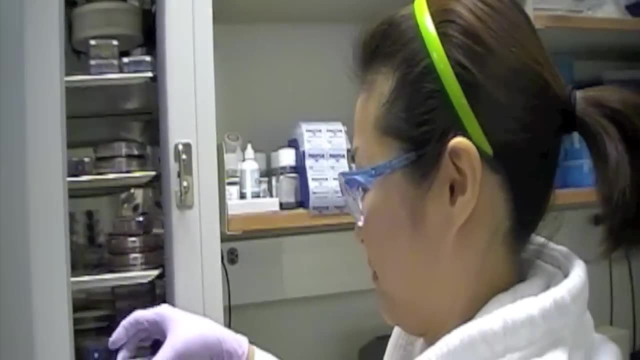 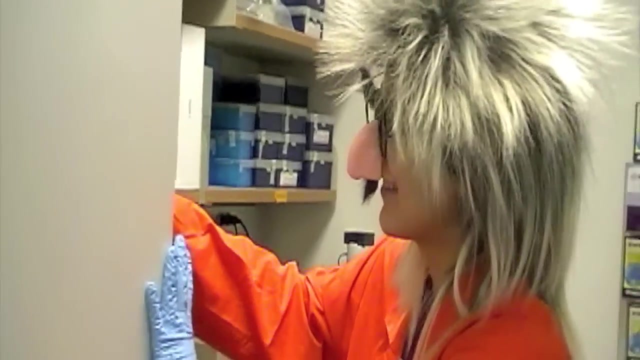 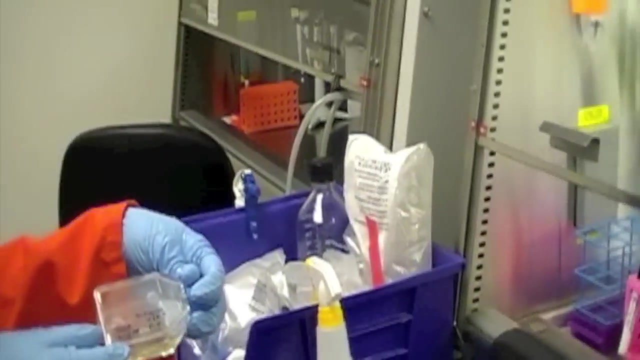 So, once all your reagents are warmed up and inside your hood, you are ready to start. Get your cells from the incubator and notice that Dr Klin is wearing gloves all the time And Dr Contamination. what is that inside your mask? 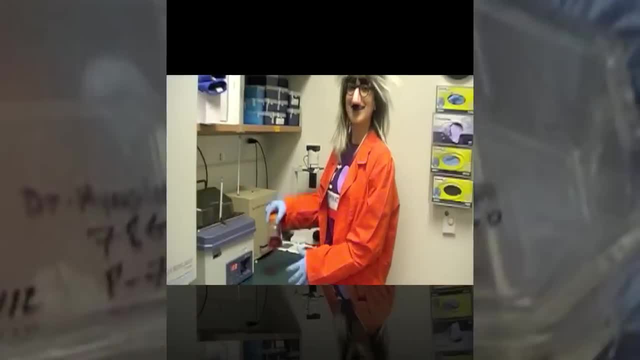 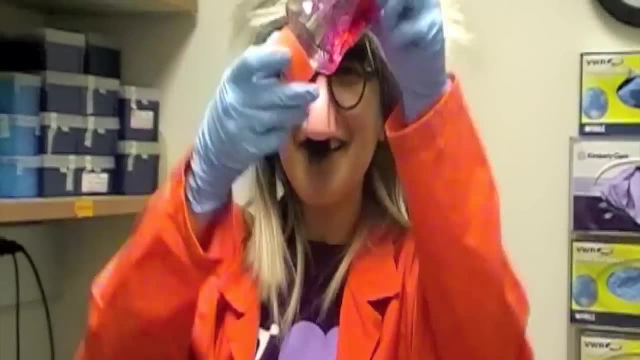 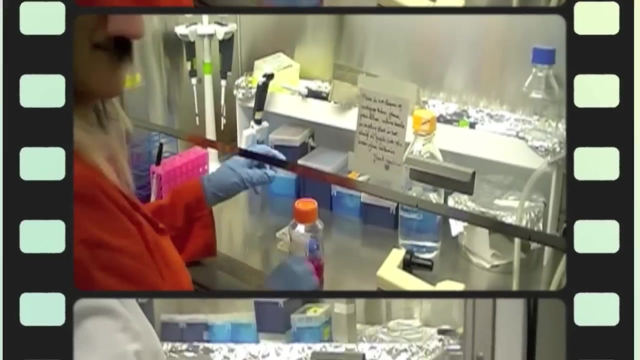 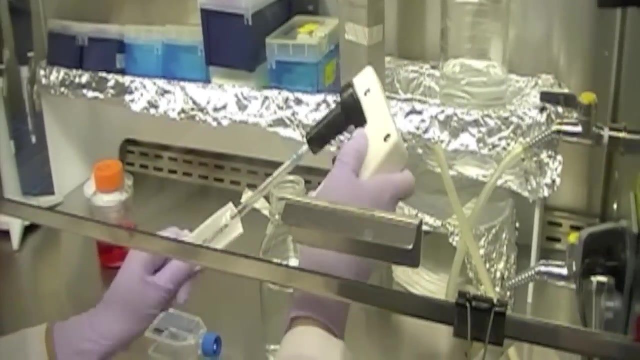 Gungus Disgusting. And don't tilt your bottle like that. Ugh, Clean your bottle better. The first step when passing your cells is to aspirate the media out of the flask and add about 2 mL of PBS to the flask. 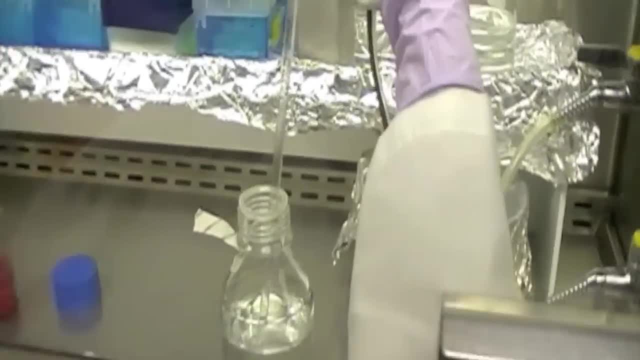 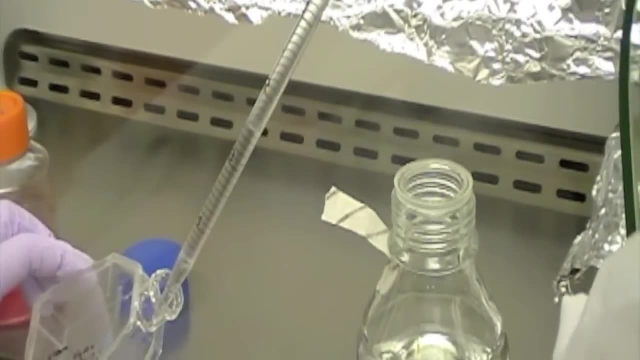 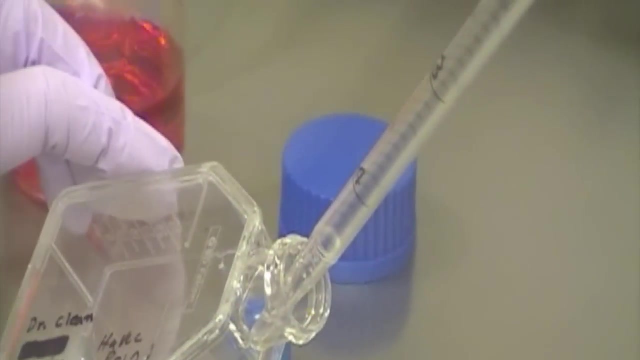 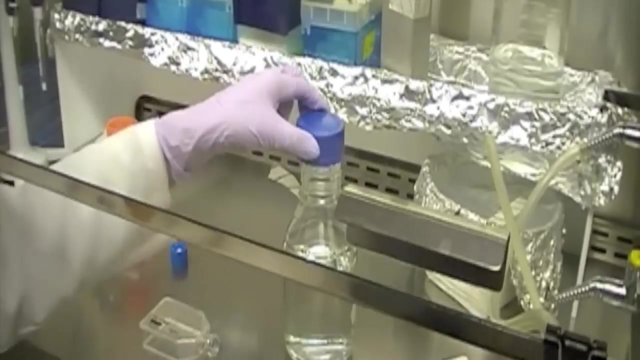 Notice how careful Dr Klin is and how careful she is And how she avoids touching anything with the tip of the pipette. Also, close the bottles right after use to avoid any dust particles falling inside the sterile PBS bottle. Gently swirl the flask to wash all the cells with PBS. 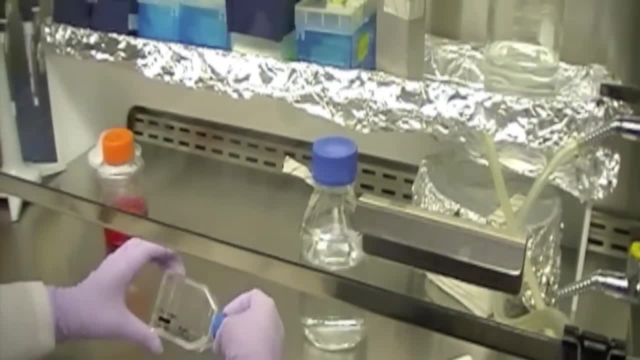 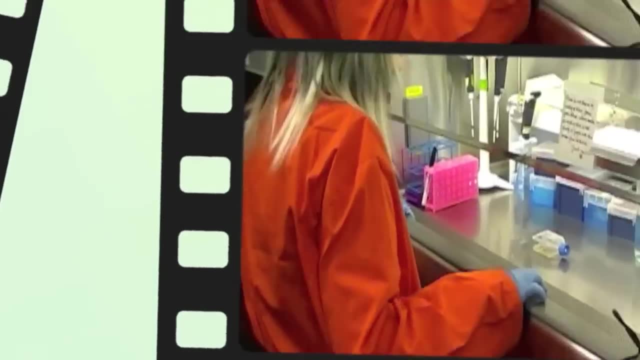 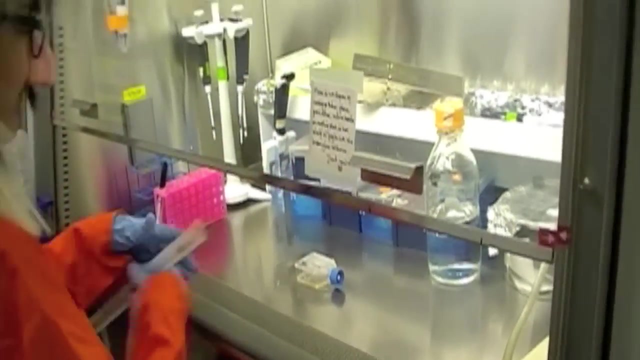 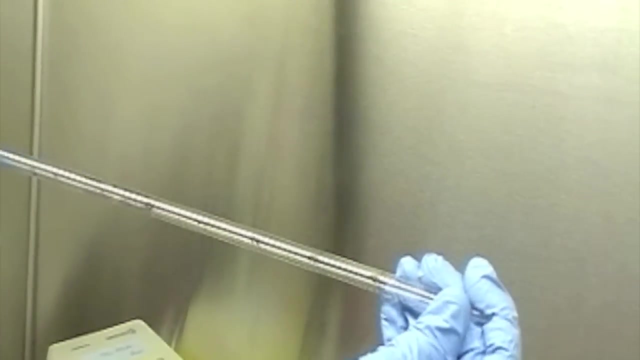 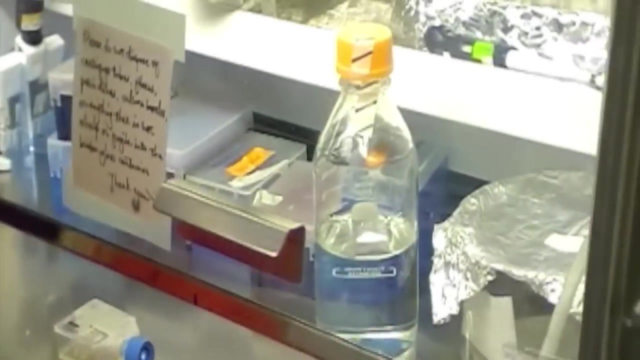 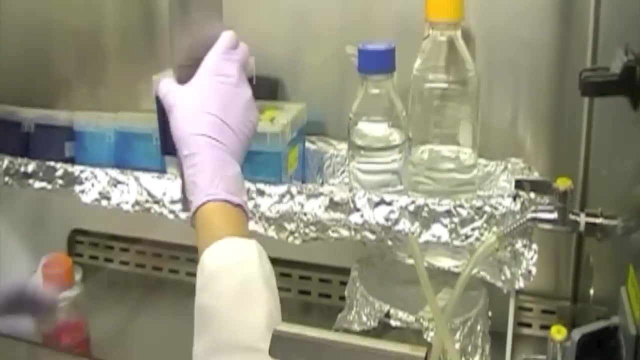 And make sure you open the pipette through the top and not through the tip. It's not a good practice to touch the pipette with your fingers either. Always grab the pipette using the plastic wrap around the pipette. So now it's time to aspirate the PBS out of the flask. 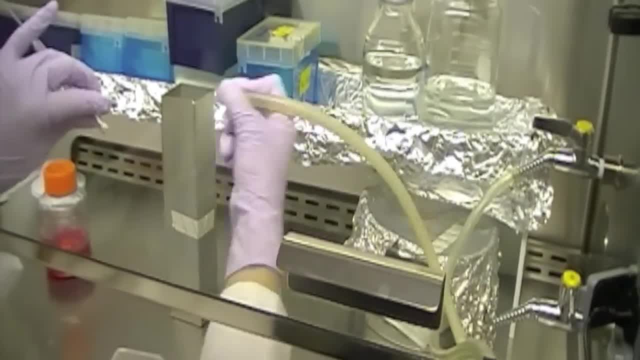 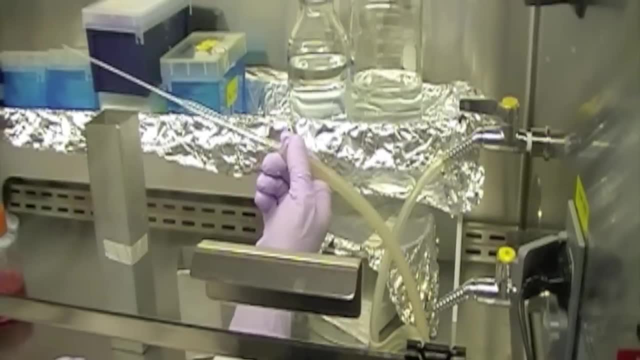 Do that by carefully grabbing only one past your pipette and placing it in the vacuum line. Tilt the flask and aspirate the PBS. The PBS wash is very important because it removes the serum in the cell culture. The serum deactivates trypsin and if we don't remove it with PBS, 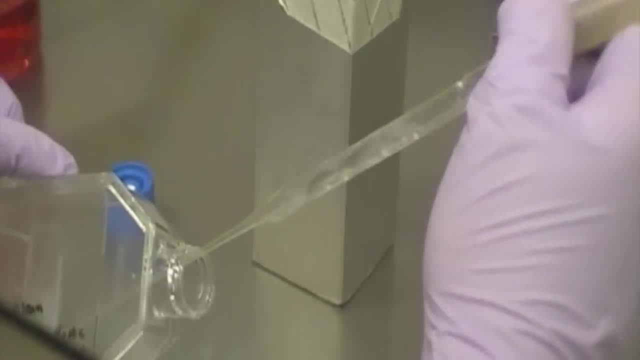 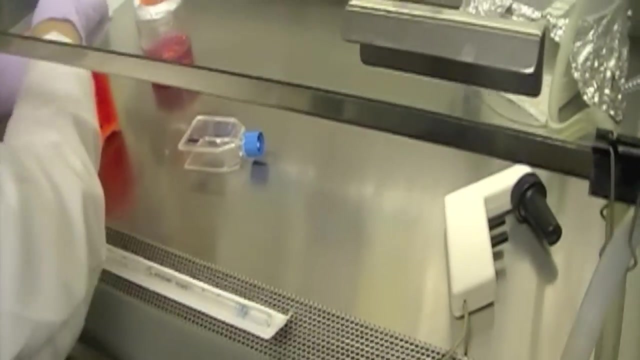 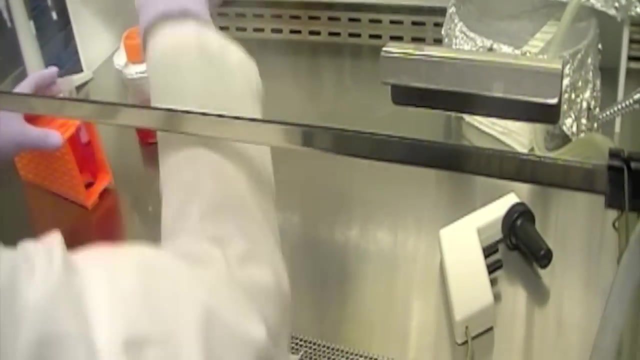 the trypsin will not work and the cells will not detach from the flask surface. The next step after washing with PBS is adding trypsin. For a T25 flask, Dr Klin will add about 1 mL of trypsin to detach the cells from the bottom of the flask. 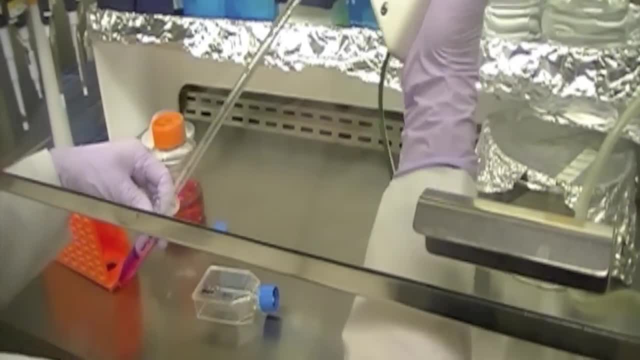 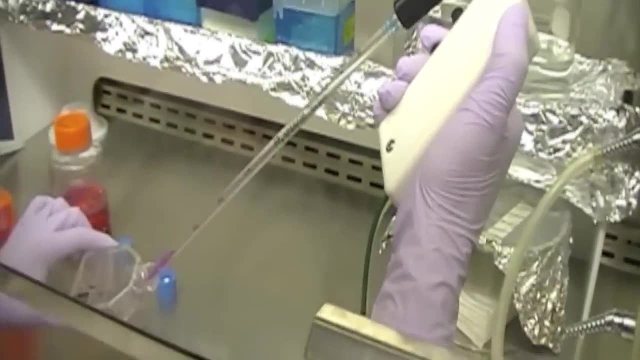 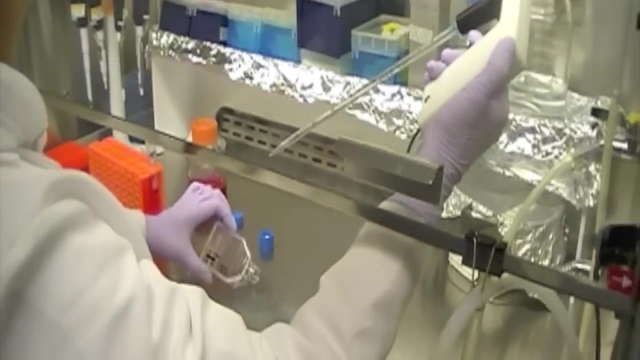 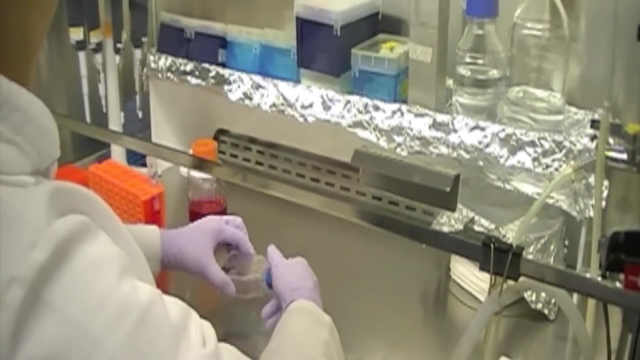 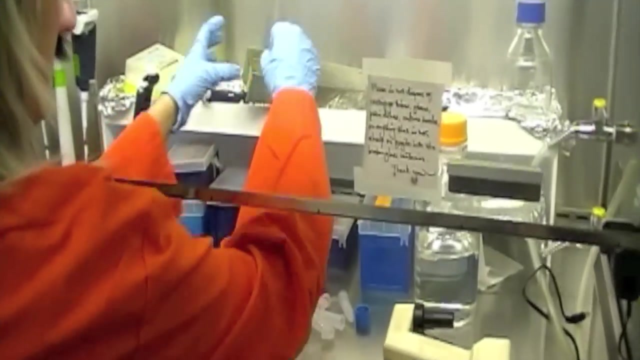 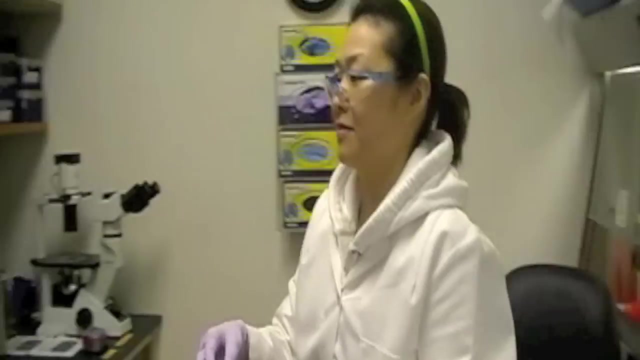 Notice how Dr Klin grabs the tube with trypsin and avoids touching the surface of the pipette. She also closes every bottle after use And remember to touch only one pipette After the trypsin has been added to the flask. incubate the cells. 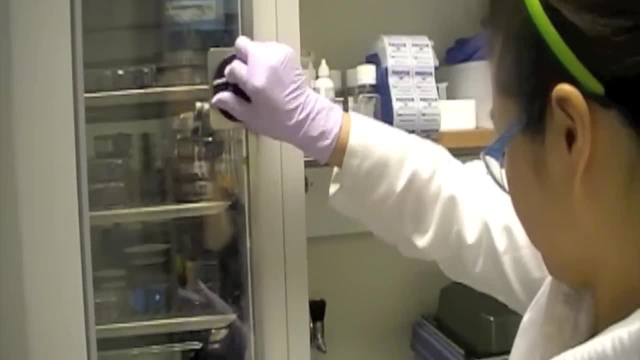 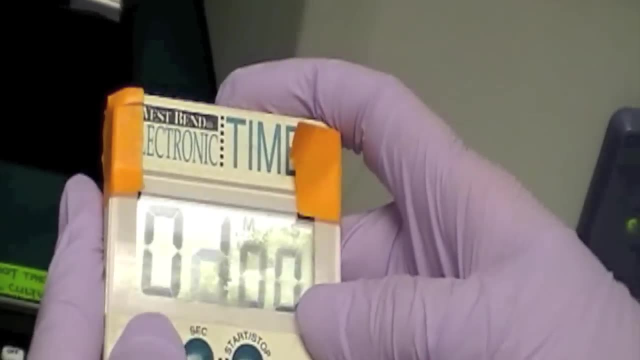 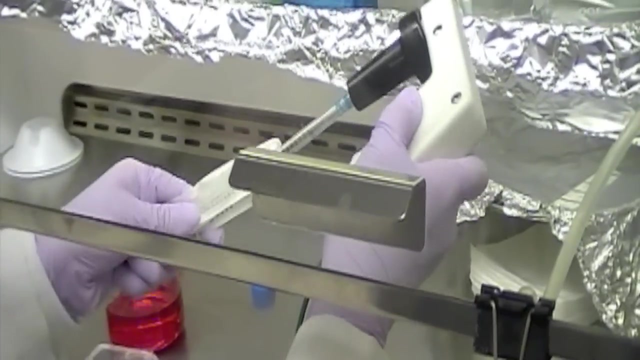 In this example, the cells will be trypsinized for 3 minutes. Every cell passage protocol is different, so you might have to trypsinize your cells for longer or shorter depending on the cell type. After trypsinizing your cells, we're going to resuspend the cells in media. 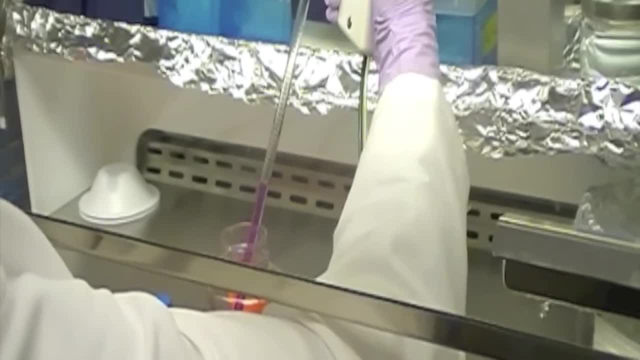 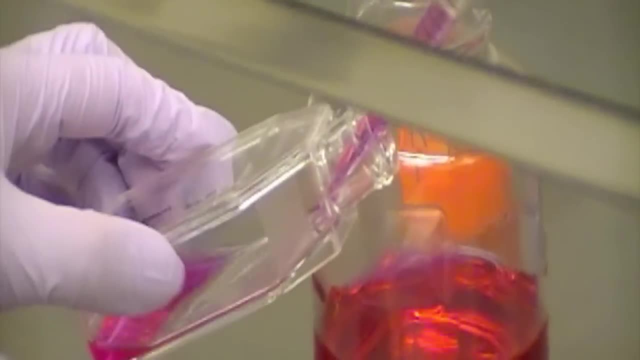 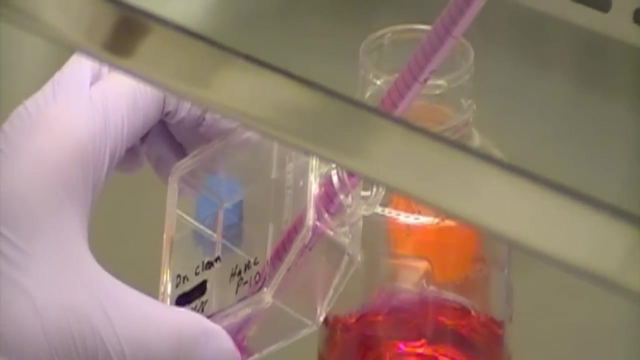 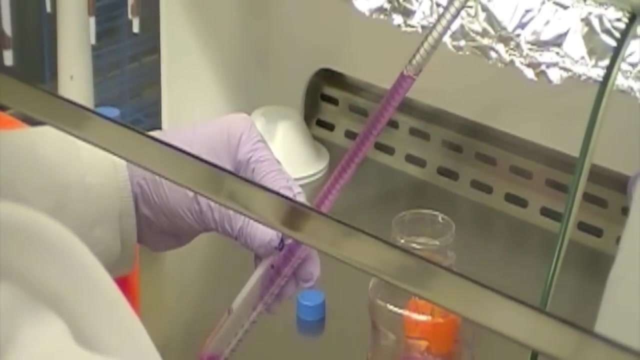 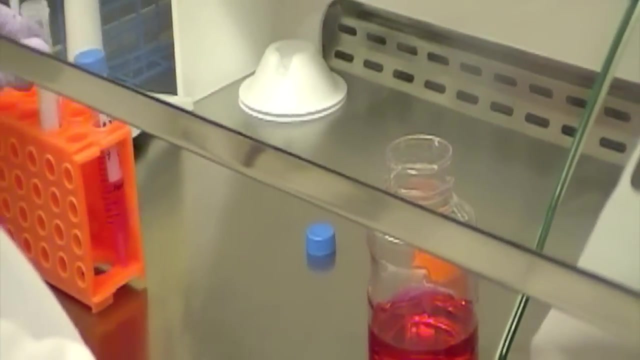 Add about 5 mL of media and resuspend by mixing the cells up and down with the pipette. Do this gently, Collect all the media and transfer it to a separate centrifuge tube. Since this pipette has been contaminated with cells, we will dispose of it inside the plastic bleach-containing pipette disposer. 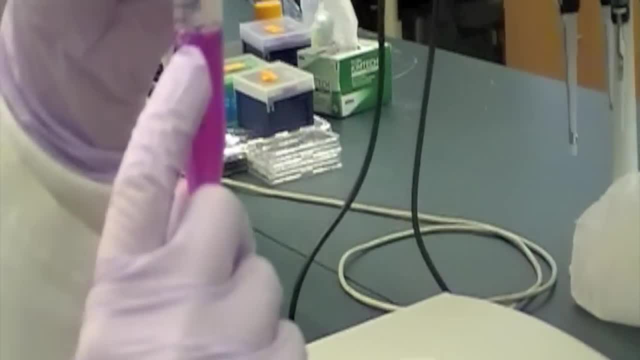 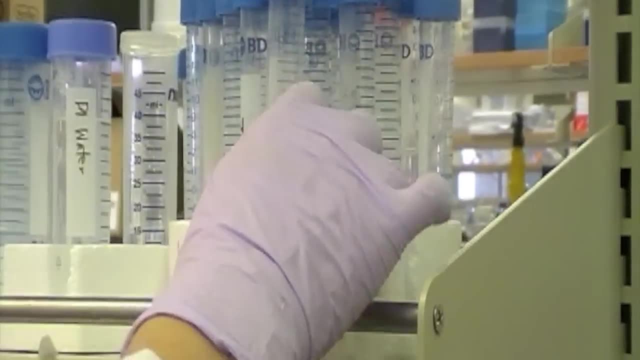 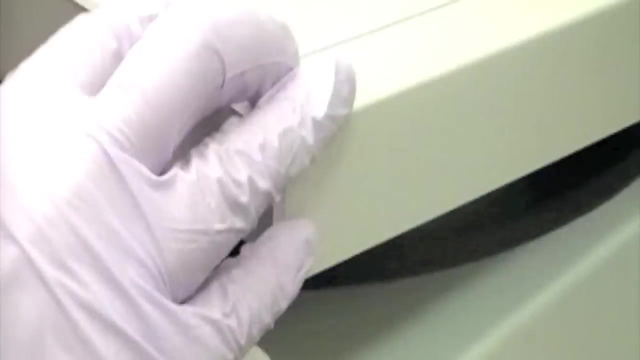 Now for centrifuging cells. we will use the centrifuge outside the cell culture room and counterbalance it with a tube of equal volume of water. In this example, we will centrifuge the cells at 1000 rpm for 3 minutes. 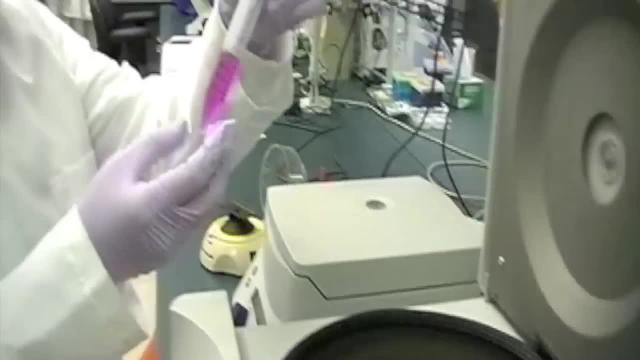 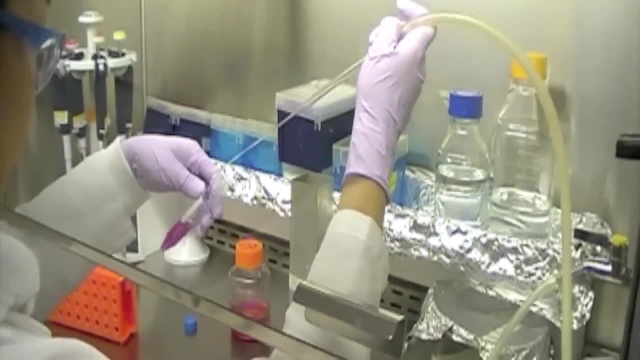 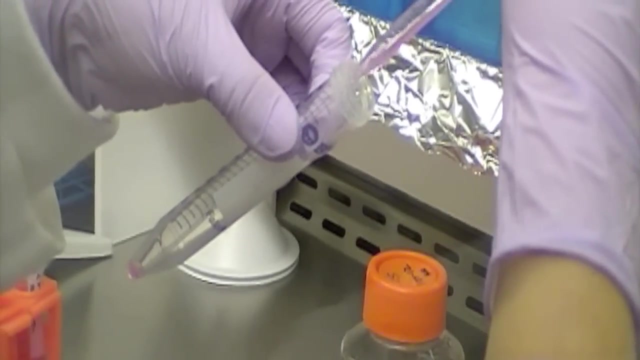 After centrifuging for 3 minutes, you will notice a pallet of cells at the bottom of the tube. After spraying the tube down with ethanol, we will carefully aspirate the media supernatant and will watch out not to aspirate the cell pallet at the bottom of the tube. 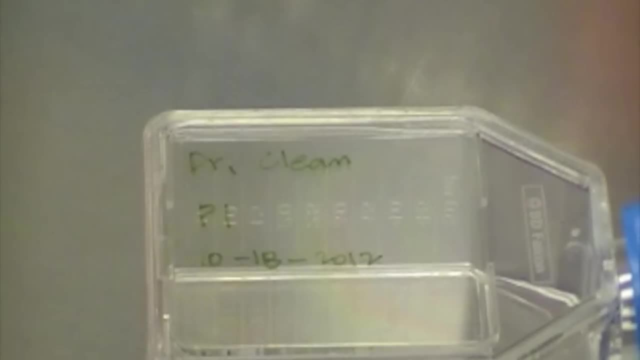 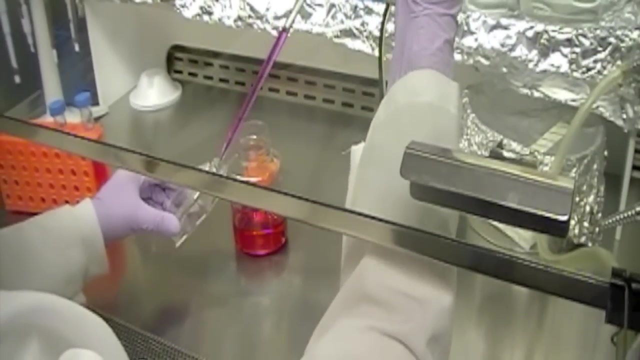 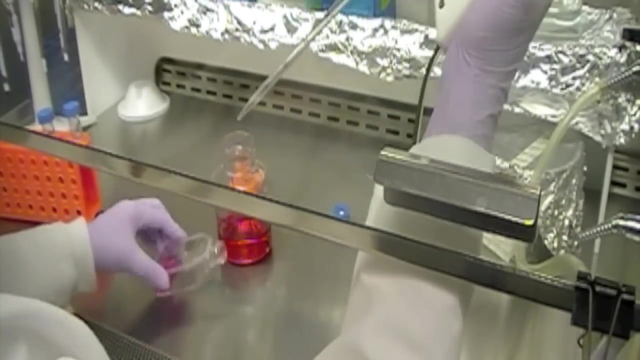 A new flask has been labeled with the cell type, passage number, date and your name. Add about 5 mL of fresh media to this new flask and dispose of the pipette in the regular cardboard box, because the pipette did not contain any cells. 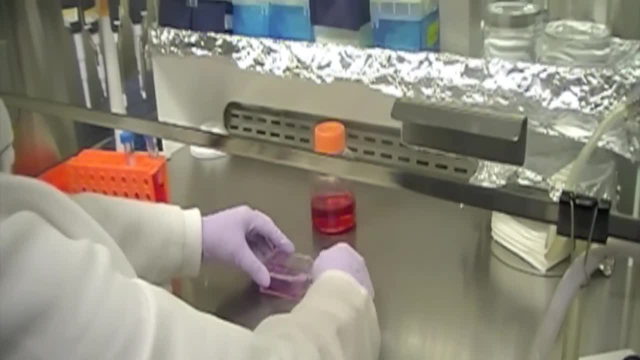 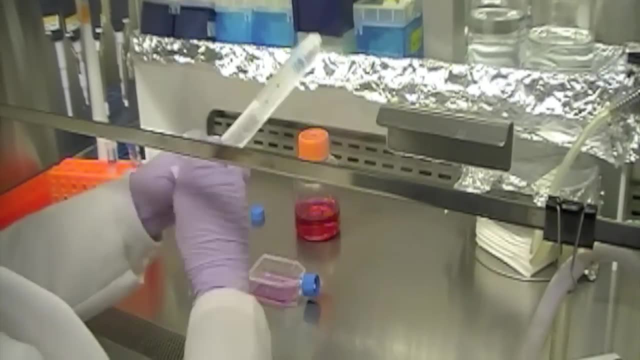 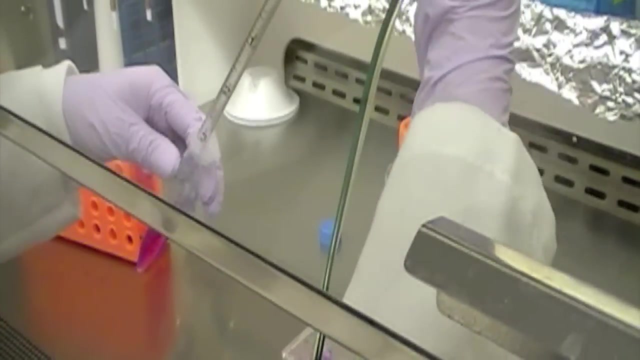 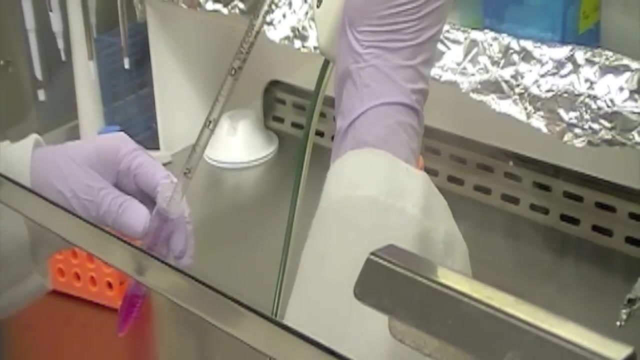 Swirl the flask with the media to cover the inside surface of the flask and finally resuspend your cell suspension by mixing up and down with the pipette. For this example, 1.5 mL will be added to the new flask, out of a total of 6 mL of cell suspension to perform a 1 to 4 passage ratio. 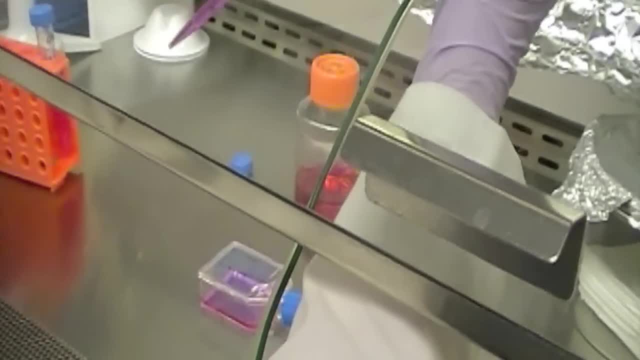 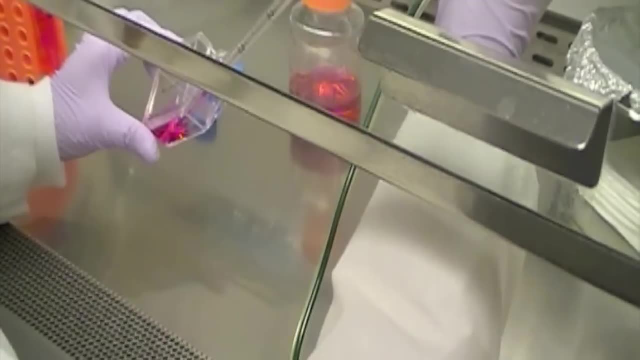 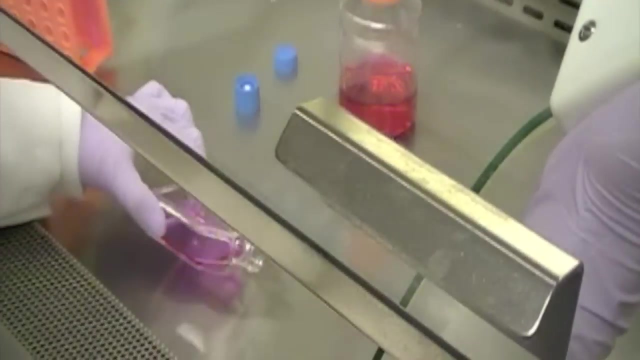 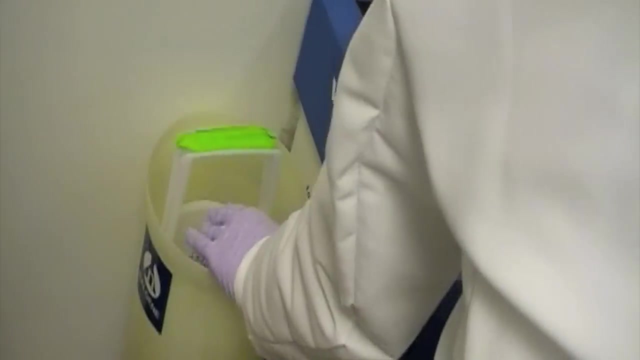 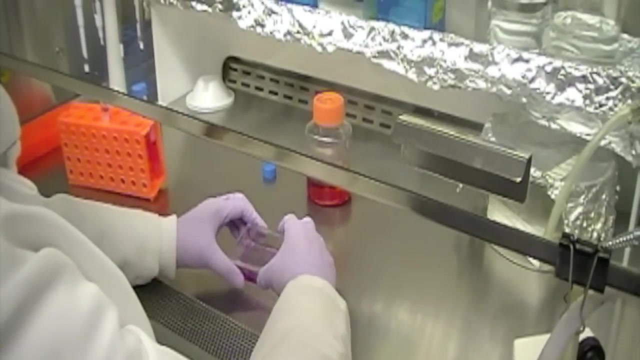 Once again, different cell lines grow at different rates and the passage ratio will vary according to the cell type. Ask someone in lab or check online to find out what is the correct passage ratio for your specific cell line. Finally, gently swirl the flask to make sure the cells are distributed homogeneously in the flask.